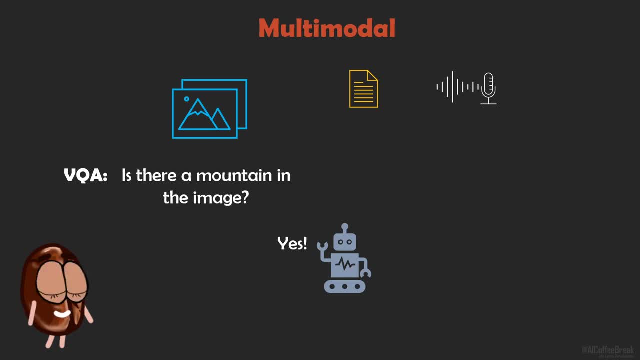 applications, especially for visually impaired people. Text-to-speech is another application, where the computer reads something out loud for us, Or vice versa in speech-to-text, where we dictate something to the computer. These were just some conventional applications of multimodal machine learning. They can also. 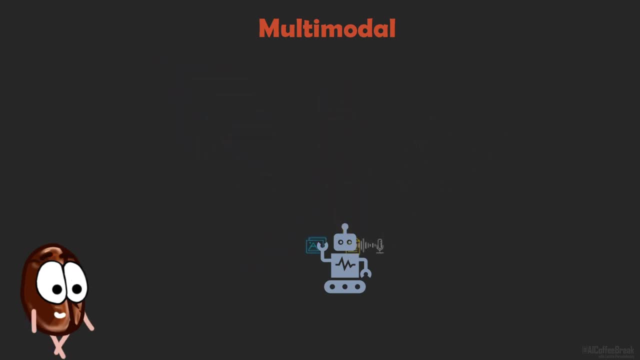 get as creative as one can think of spanning other modalities than just text messages or speech, like humidity levels, pressure, depth data. The pressing question now is what makes these input signals different enough so we can treat them as different modalities. 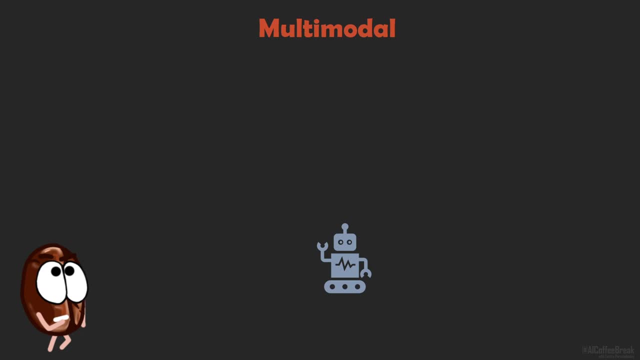 and not just like more data of the same kind. What makes these input signals different enough so we can treat them as different modalities and not just like more data of the same kind? What makes these input signals different enough so we can treat them as different modalities? 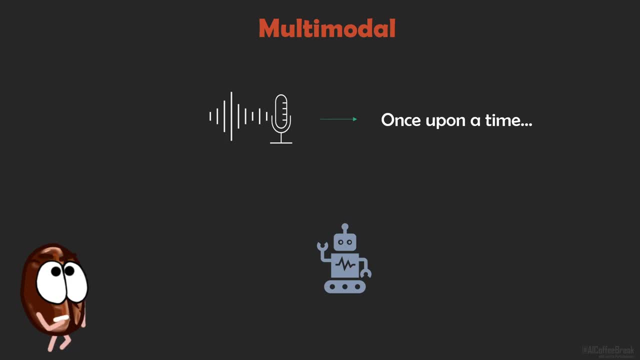 and not just like more data of the same kind. What makes these input signals different enough so we can treat them as different modalities and not just like more data of the same kind? But since we put it like that, are text and speech not just the same modality- Speech. 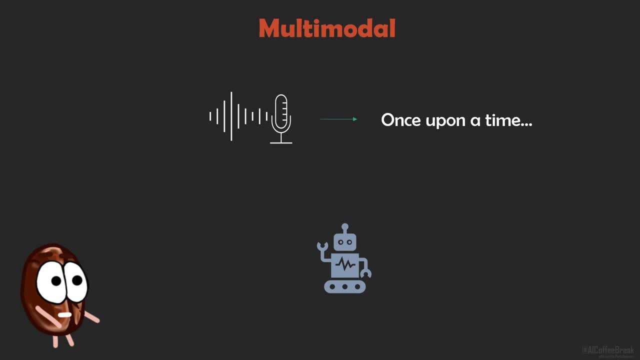 transcribes to text and can be read out loud and become speech, right? No, wait a little. Speech contains paraverbal information. if we want to sound intelligent, or in simple words, speech contains much more than text, like intonation, very subtle voice modulations. 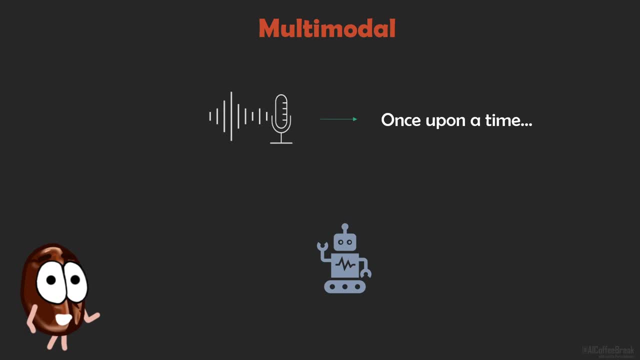 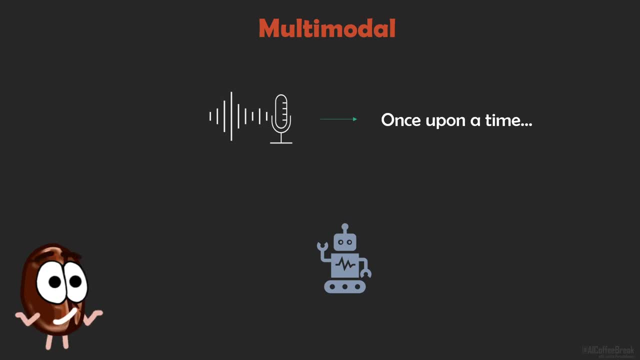 is not captured by a pure transcription. Okay, okay, one more chance. What about text and a picture of the same text? Are they not the same modalities? even though one is text and one is an image of the same text, They contain the same information, right? 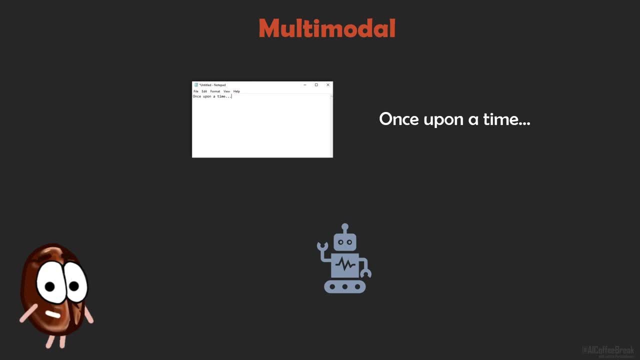 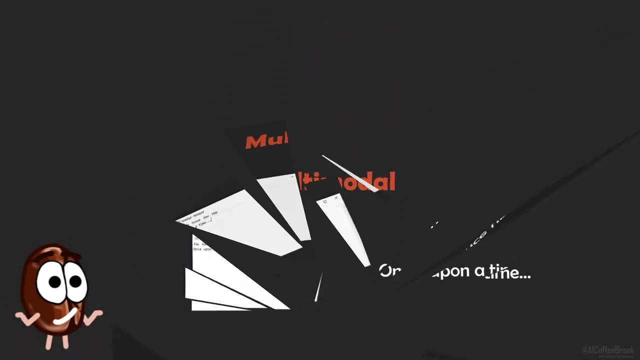 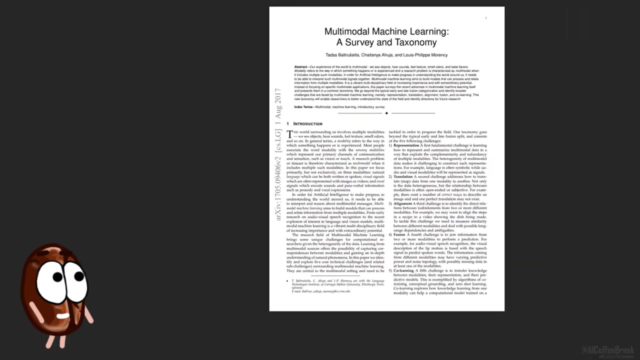 Well, here we are with some questions that Ms Coffee Bean kept asking herself and started to search for what others could be say about this matter And where to look if not at surveys written by experts in the field. One survey paper defines multimodality already in the first lines of the abstract. 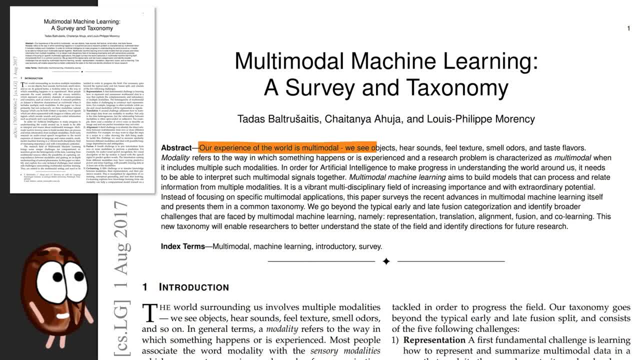 Let's see what it says. Quote: Our experience of the world is multimodal: We see objects, hear sounds, feel texture, smell, odors and taste flavors. Okay, until now one can agree. Modality refers to the way in which something happens or is experienced. 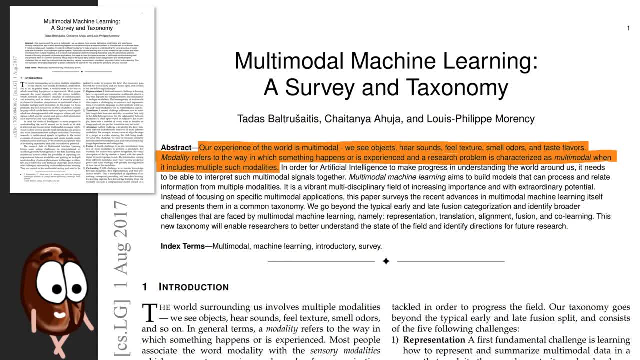 and a research problem is characterized as multimodal when it includes multiple such modalities. Hmm, Ms Coffee Bean, what do you say about this? No, This definition is definitely based on human experience and human senses to define modalities, But Ms Coffee Bean dislikes that we are talking about. 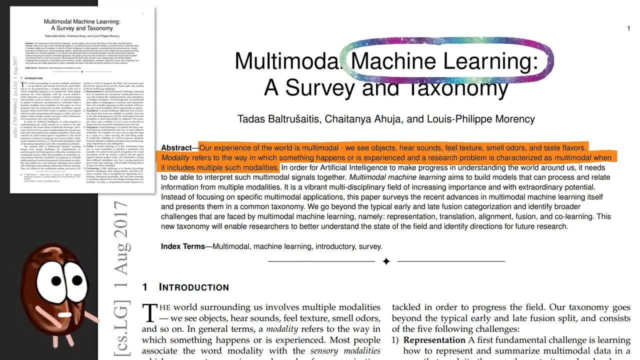 machine learning. It's in the title. So about programming machines to do things. Then why are we talking about human experience when we should perhaps focus on the machine experience? The computer is the one that has to convert text to speech, and it has to be. 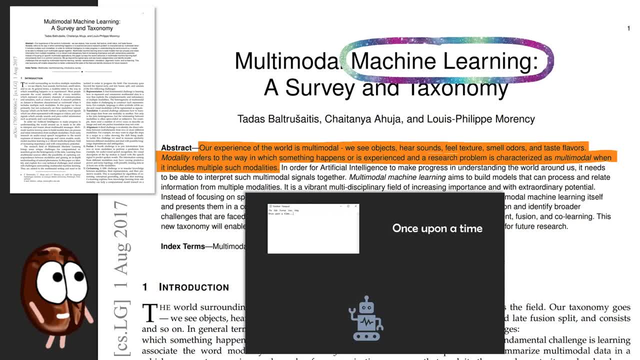 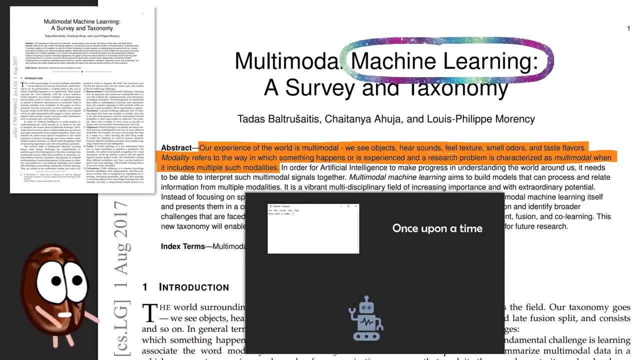 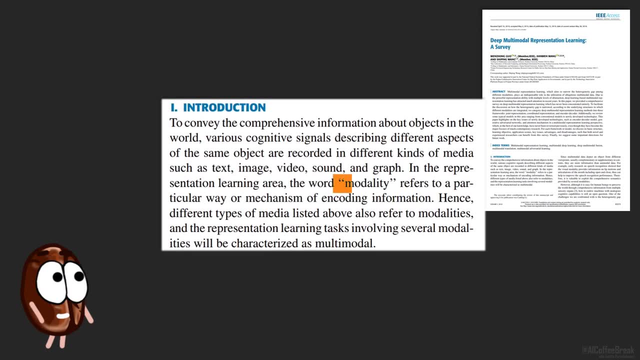 Because they are very similarly experienced by humans, Not to even start to mention other organisms than humans that experience the world completely differently, like seeing infrared or perceiving light, polarity. So let's see another informed opinion. Modality refers to a particular way or mechanism of encoding information. 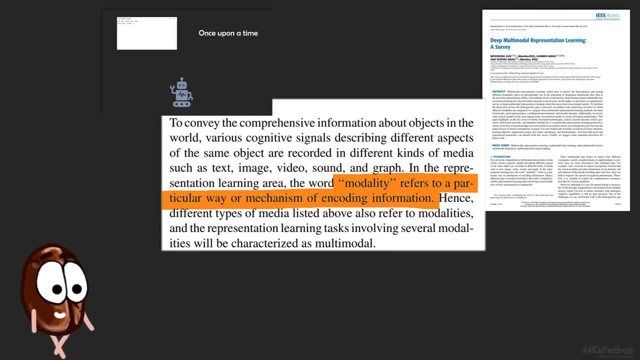 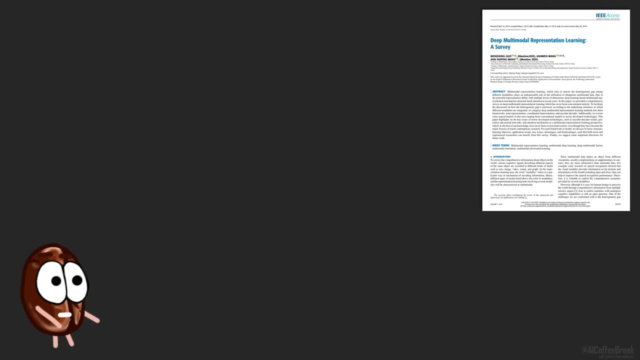 After this definition, a text in a text file and a screenshot of that text are different ways to encode the same information, so there are different modalities. This might upset the human in us, but it makes sense for a machine that does not know that the text in the image represents the. 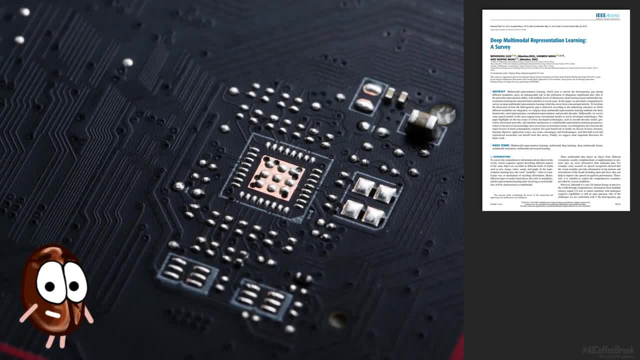 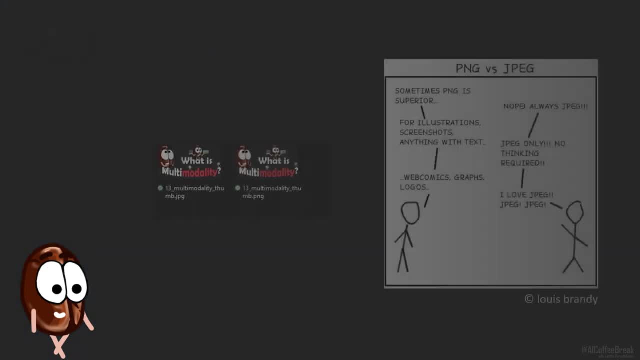 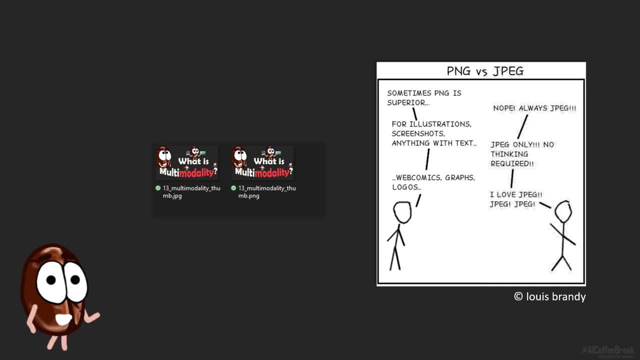 same thing. The machine usually knows only about 0 and 1s, and the rest is programming. But after this definition, JPEG and PNG are different modalities too, because they are different ways to encode the same information of any image. So what is happening here? 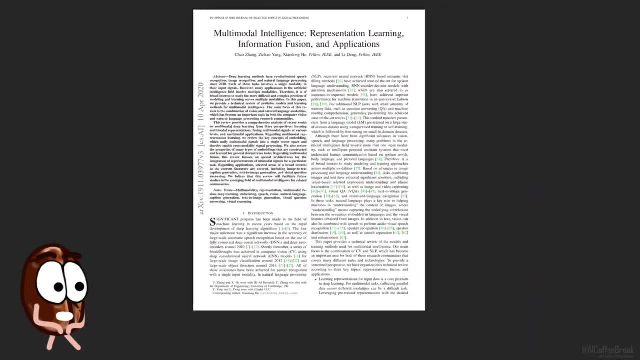 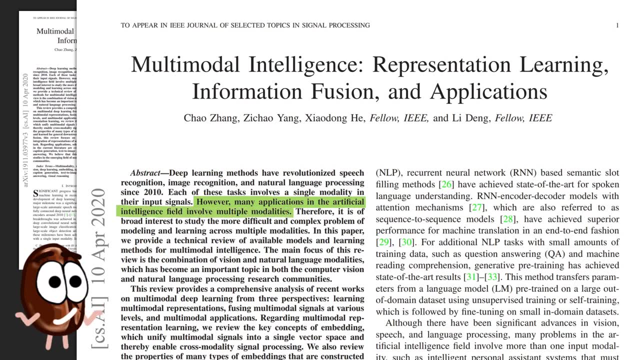 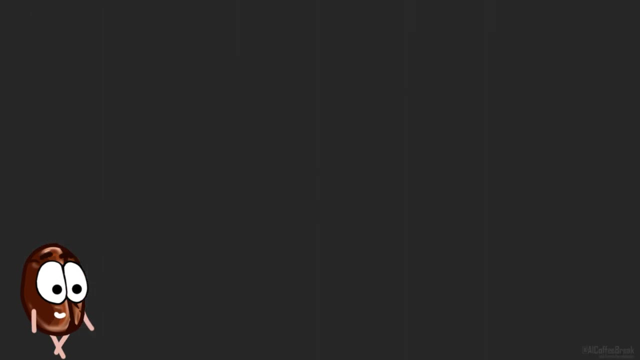 Other surveys about multimodal intelligence ignore the definition of multimodality altogether, or they define multimodality by stating that multiple modalities are involved. Multi-modality- It's in the word. To put it in a different way, When talking about the word. 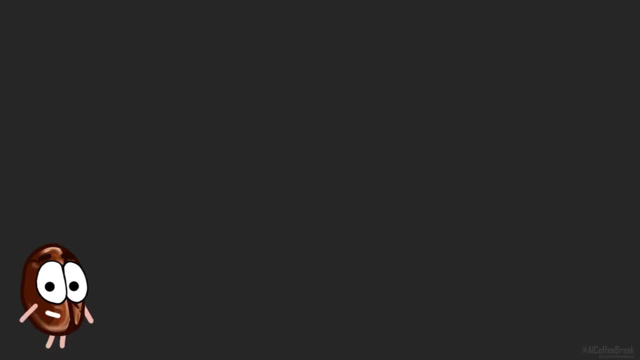 modality. many speak about it like everybody knows what it means, but actually nobody knows what it really means. So what is the difference between multimodality and multimodality? I think it's time to sort this a little In all the surveys and papers we read. 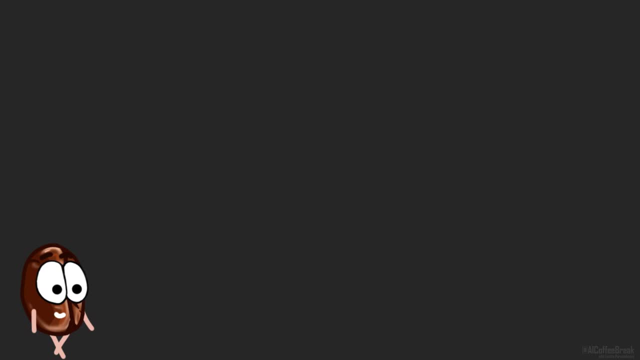 we found either definitions of multimodality related to senses and experiences- to taste, smell, vision, hearing- which we will call human-centric. We also found a media or data-type related definition, considering images, text, graphs as being different modalities. These 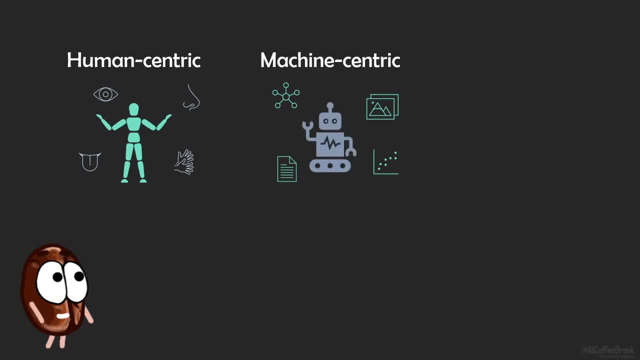 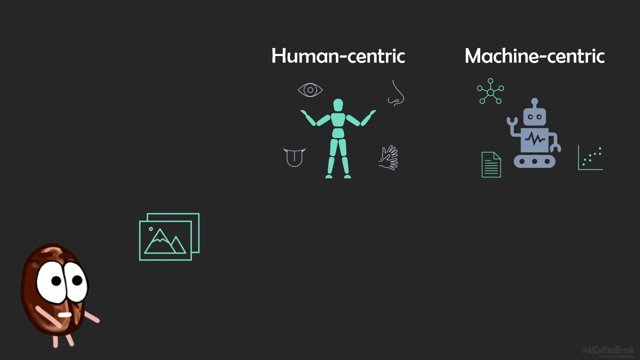 definitions we will call machine-centric. We also found an etymological definition of multimodality, which we will call… a no, we will just discard it. Now it's time for our definition. We will start defining multimodality by first taking one input. 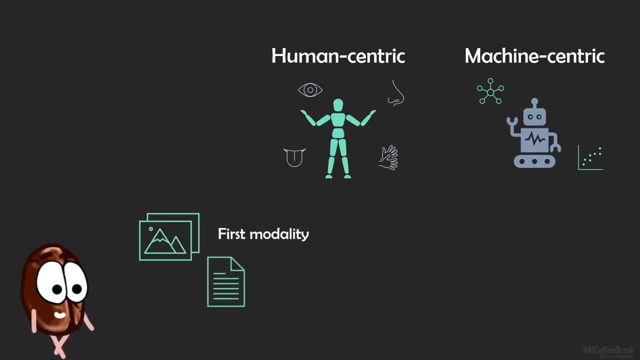 and call it the first modality. We then take a second input and ask what it needs to fulfill to be named the second modality rather than just more input of the same kind, And this is the definition we will call machine-centric. We also found an etymological definition of multimodality. 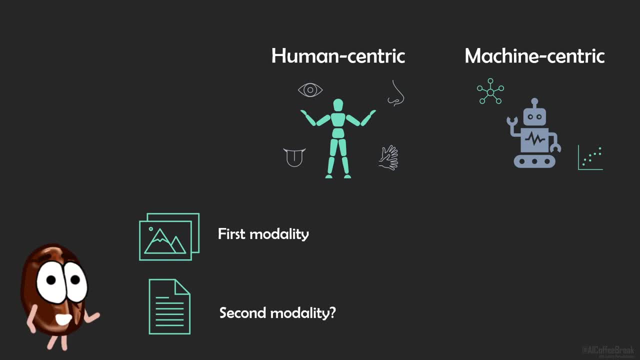 this while keeping in mind that we are talking about multimodality for machine learning. The second input might come in different encodings or formats, like PNG and JPEG, or entirely in a different data type, like a table or a graph, But when does it become a different? 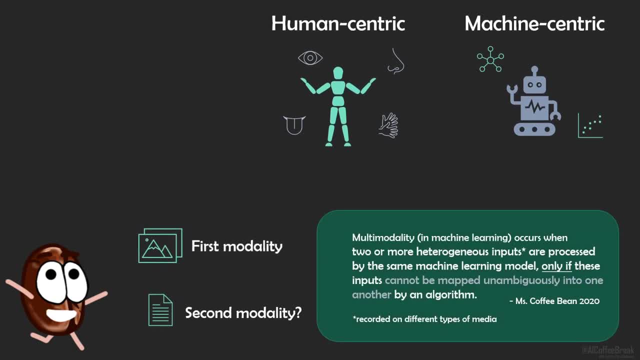 modality. We propose the following definition: We speak about multimodality in machine learning when two or more heterogeneous inputs are processed by the machine. These inputs are processed by the same machine learning model only if these inputs cannot be mapped unambiguously into one another by an algorithm. Modalities are thus not only redundant. 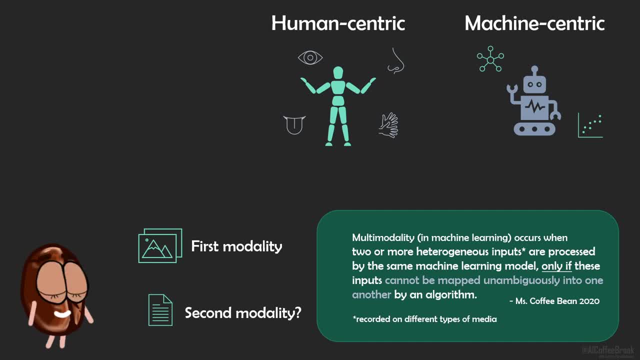 with parts that can be aligned between one another but, most importantly, also complementary, since one contains information that is not present in the other And there is no one-to-one translation between modalities. Okay, this definition just needs a name, and we are done. How about the complementarity principle Or the information-centric definition? 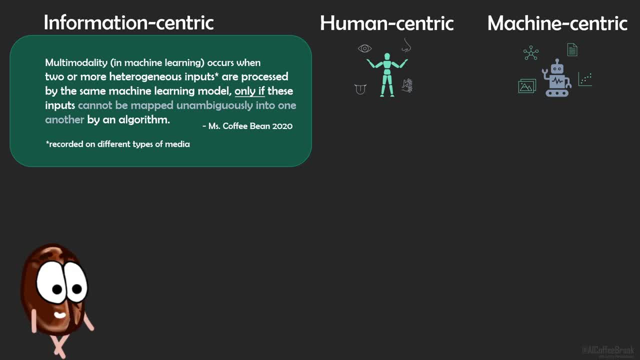 just to keep in line with the other namings. Then let's see how these definitions fare with Ms Coffee Bean's questions. Are JPEG and PNG the same modality? In our view, yes, since they can be converted into one another with a well-known algorithm. 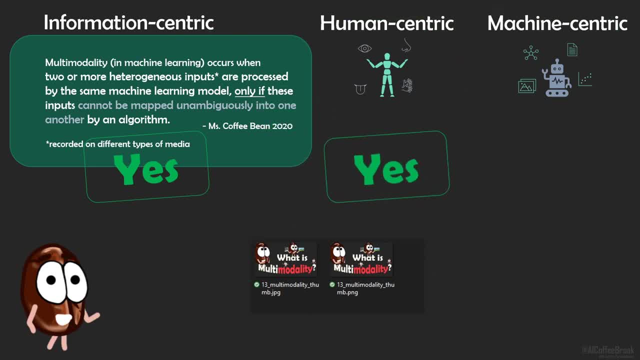 In the human-centric view they are also the same modality, since humans do not really care if the image is JPEG or PNG. For the machine it is not the same. since PNG and JPEG are different encodings, Are text and image of that text the same modality? 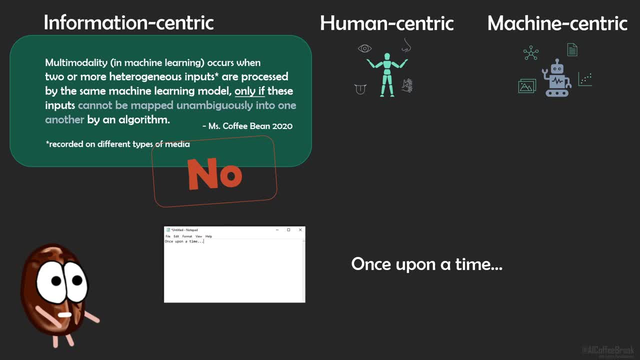 In our definition they are not the same modality. While the mapping from the image to text can be performed unambiguously, the same text has many realizations as an image, For example, I could have written the same text on paper and taken an image of it In the human-centric. 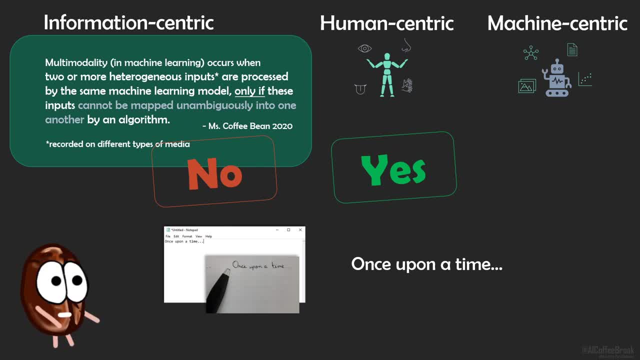 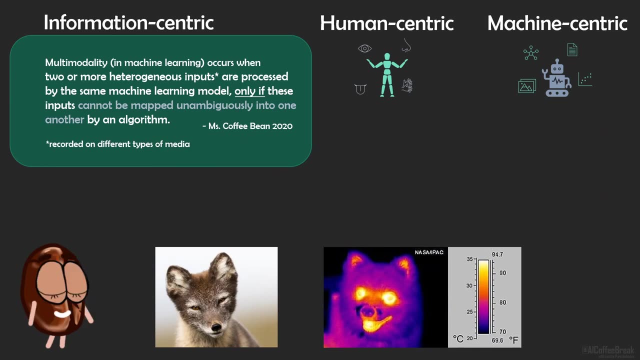 view, they are the same modality, As for us, it does not matter how the text is written, as long as we can read it. For the machine, it is not the same. since image and text formats are very different, Are RGB images and infrared the same modality? 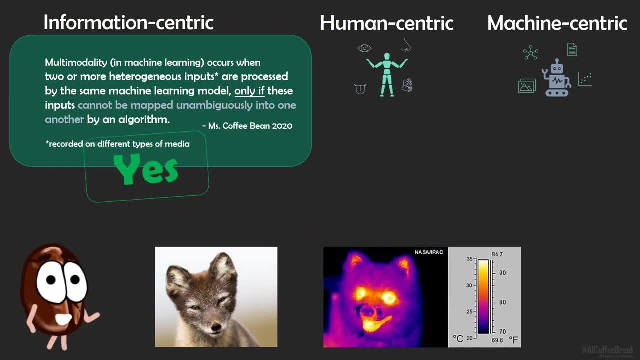 Information-centric? yes, since infrared data can be just mapped and stored into the usual red, green and blue channels. Infrared is not a different modality, but rather more data. For humans, however, it is not the same, as we do not see infrared and infrared means. 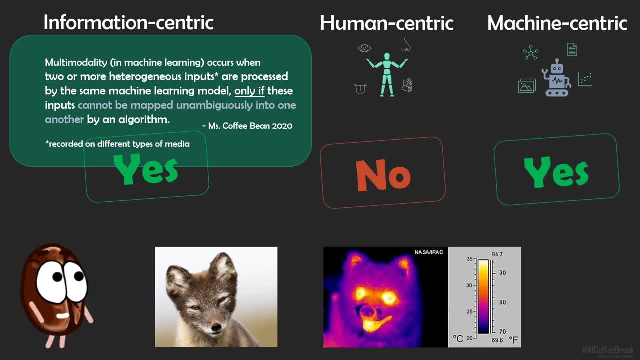 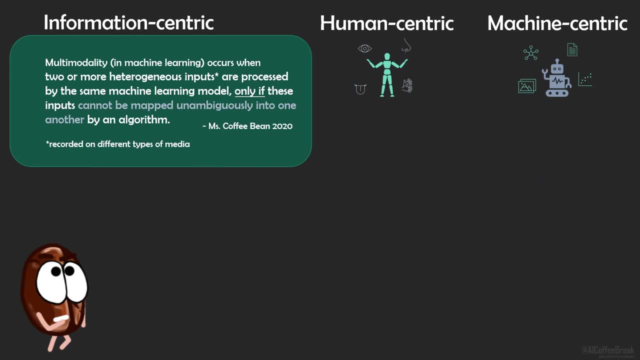 a whole new world for us. For the machine, it is the same modality if it is stored as an image. One more example: Are a graph and a table the same modality? Well, in the information-centric view, it depends what kind of graph and what kind of. 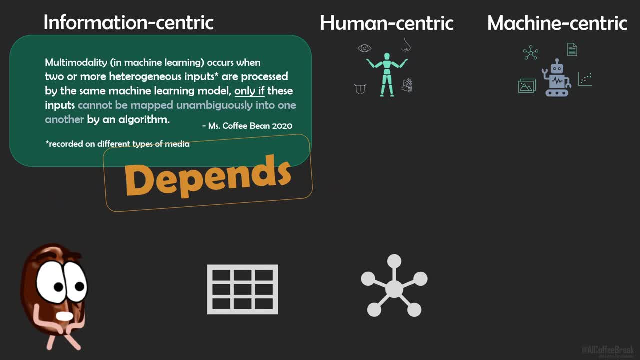 table. If the graph can be one to one-converted to the table and the table into the graph like a graph and an adjacent cell matrix, then they are the same modality. If the graph is a social connectivity graph and the